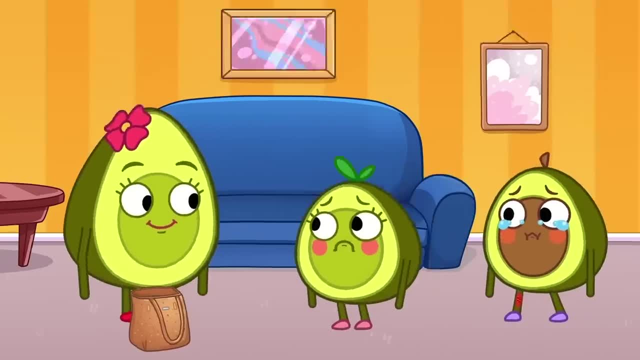 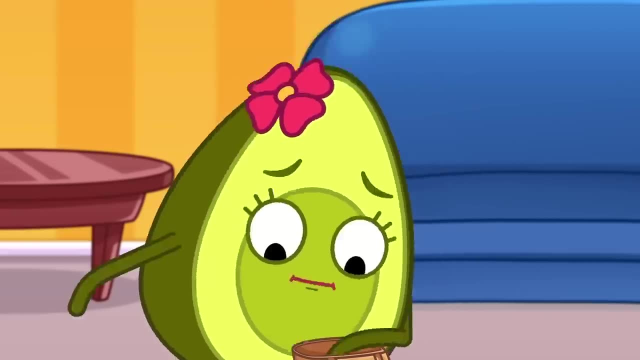 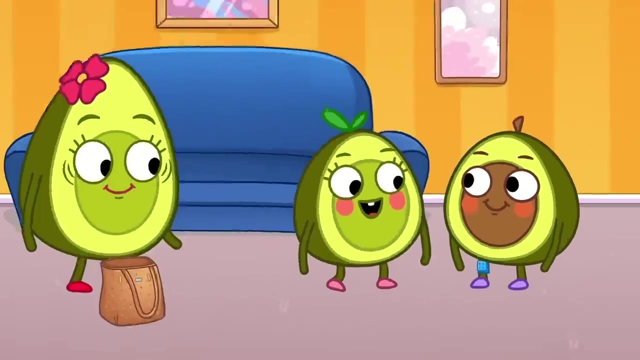 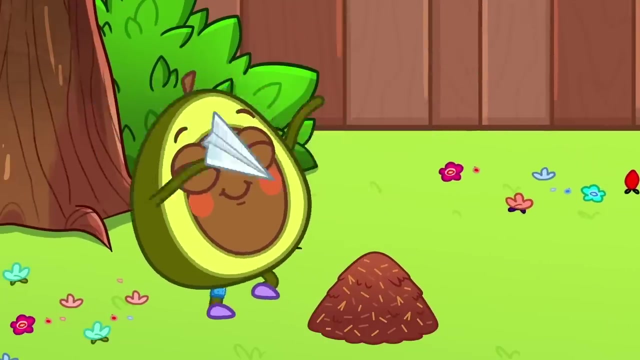 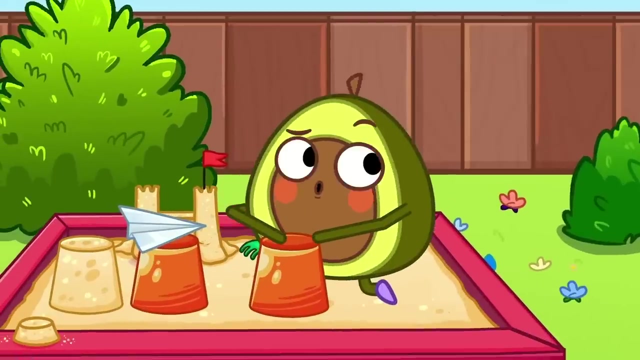 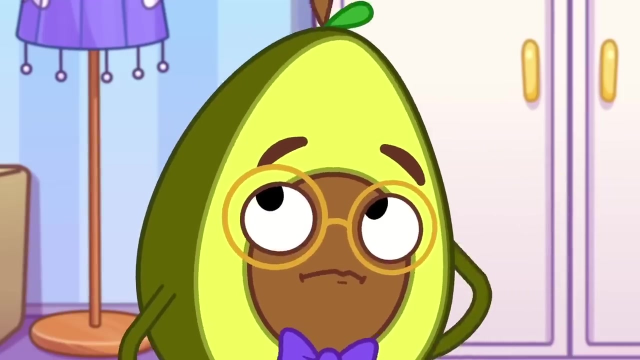 Uh-huh, Uh-huh, Uh-huh, Uh-huh. Oh, Uh-huh, Uh-huh, Uh-huh, Uh-huh. Be careful, Be careful, Uh-huh, Uh-huh, Uh-huh. 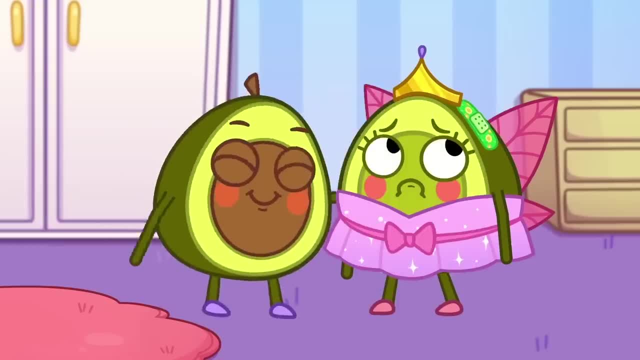 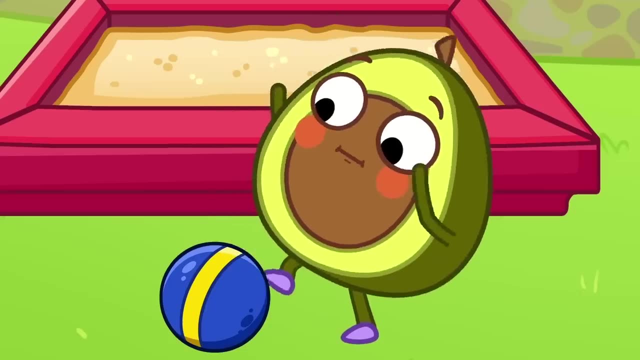 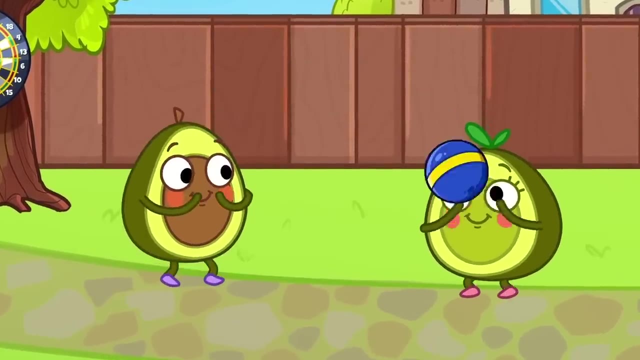 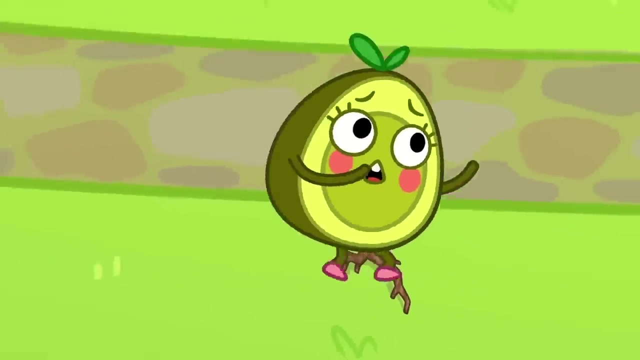 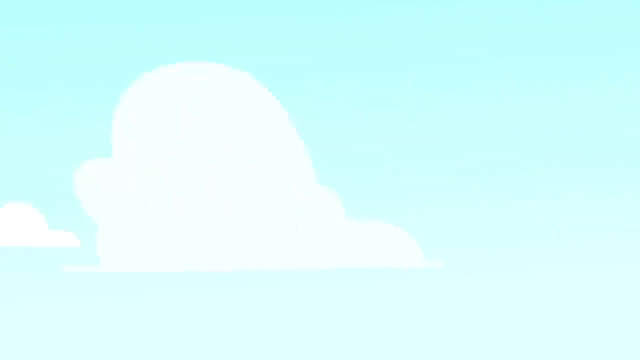 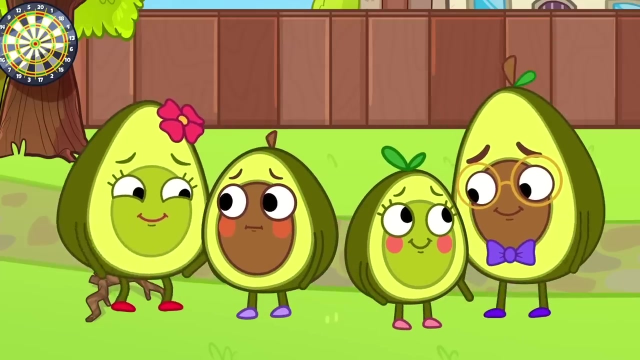 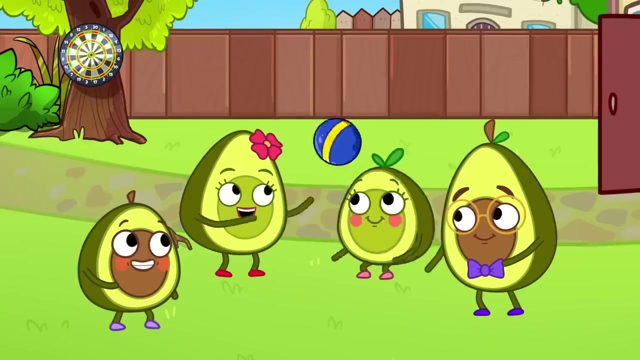 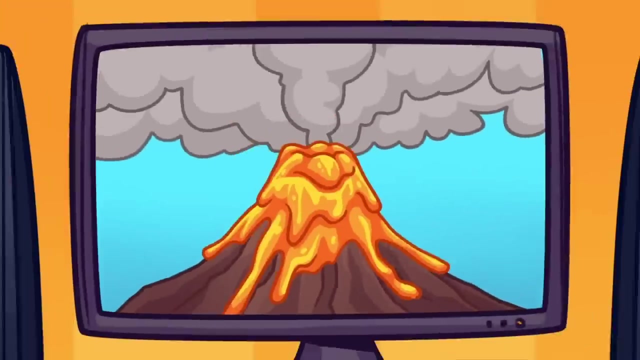 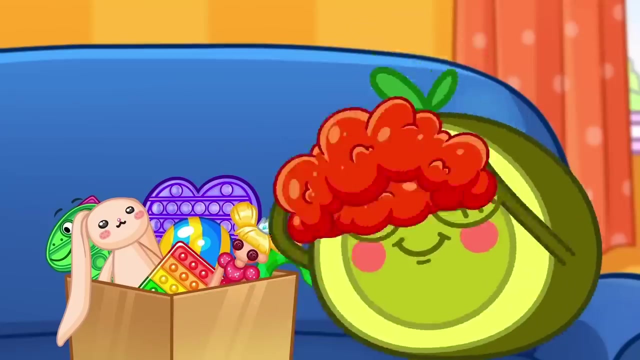 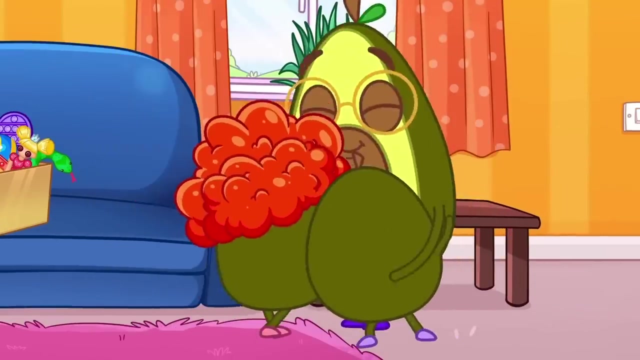 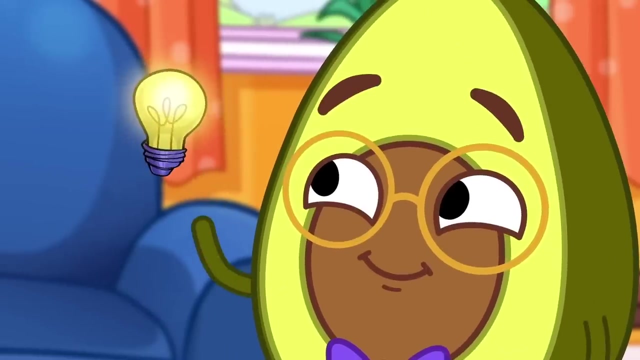 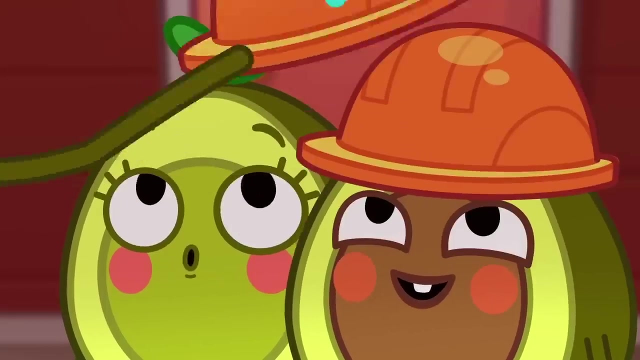 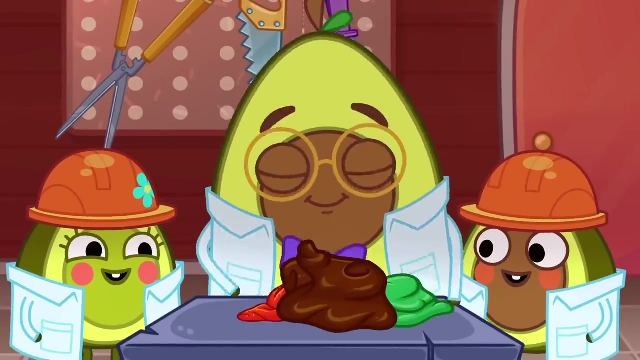 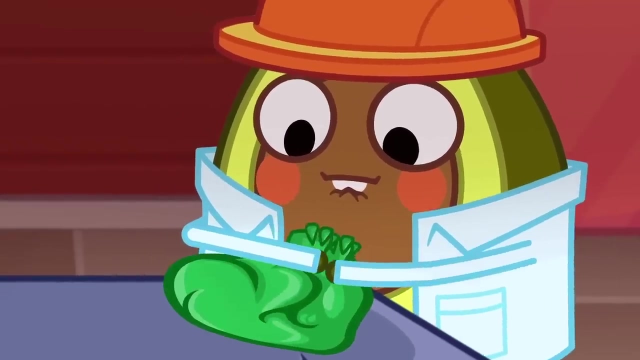 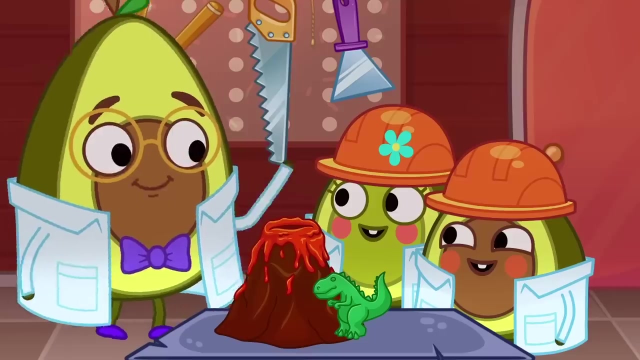 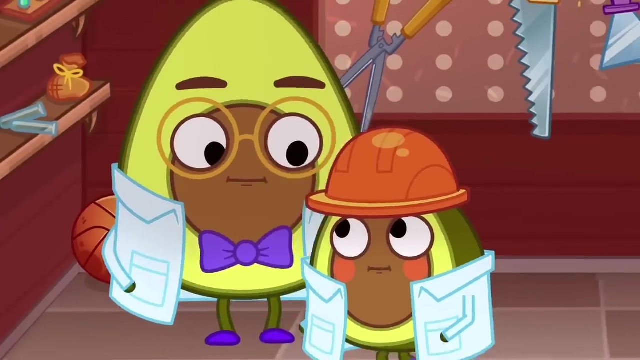 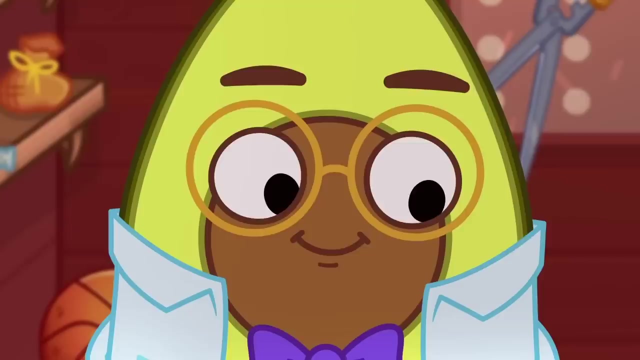 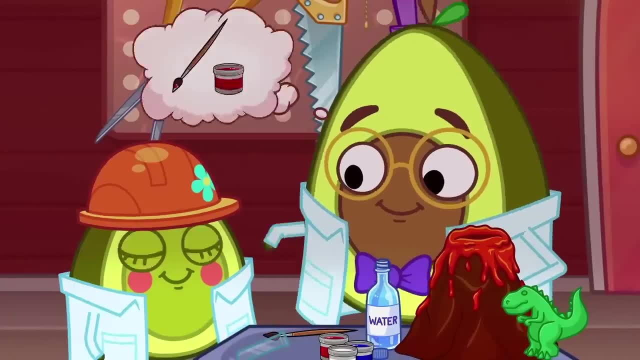 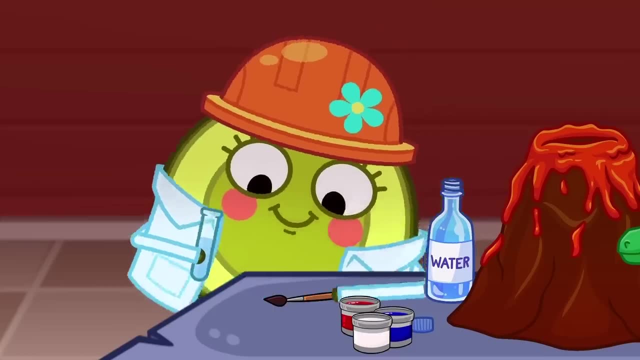 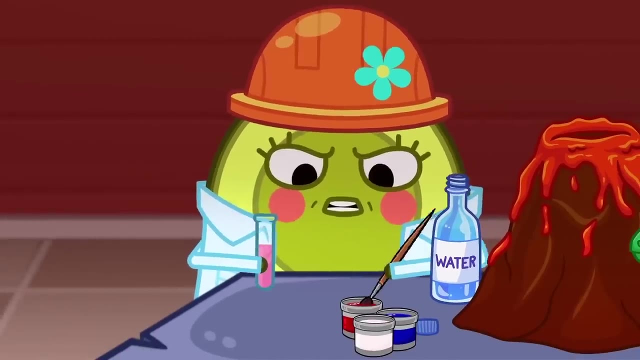 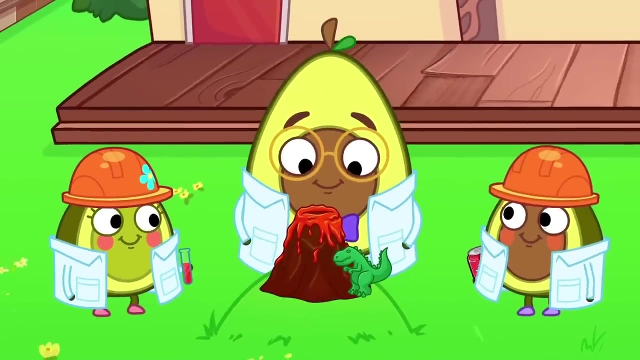 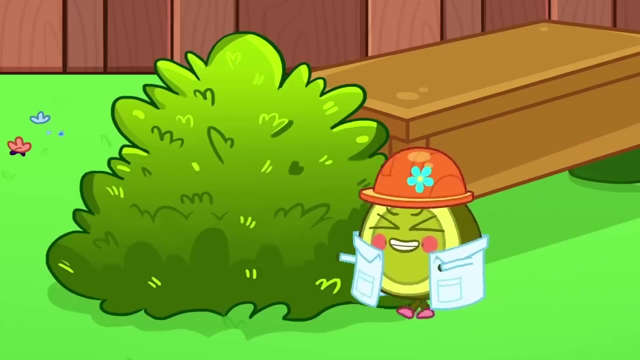 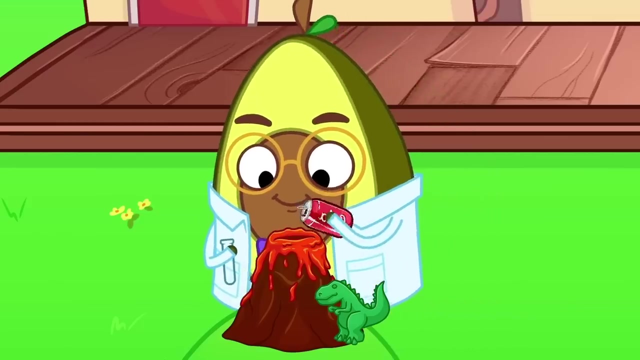 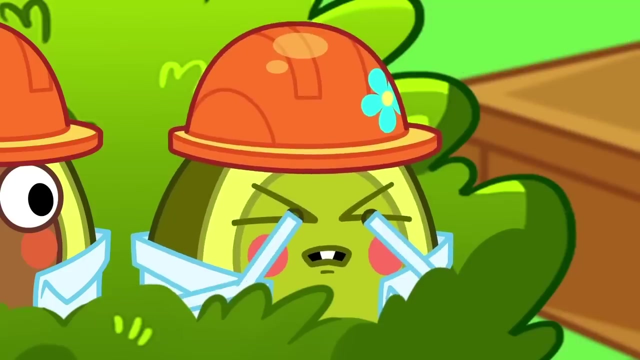 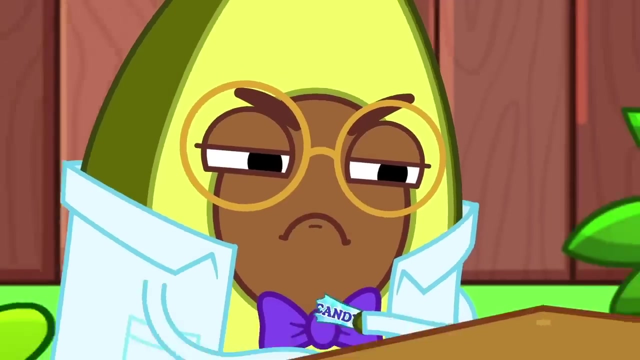 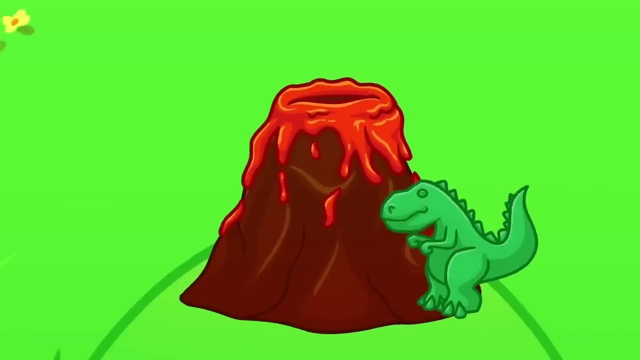 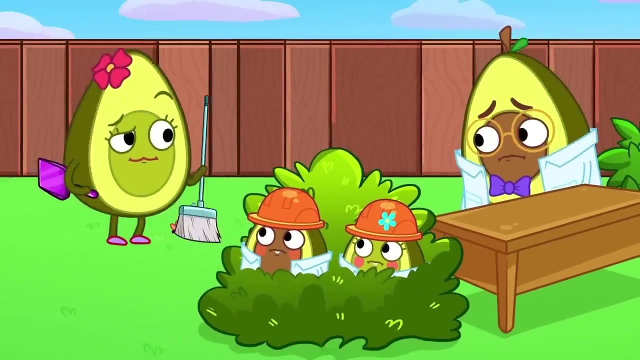 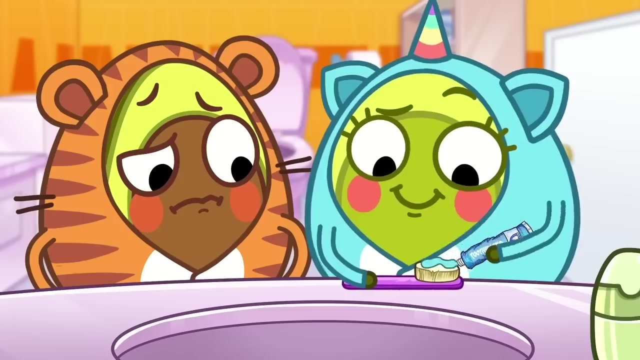 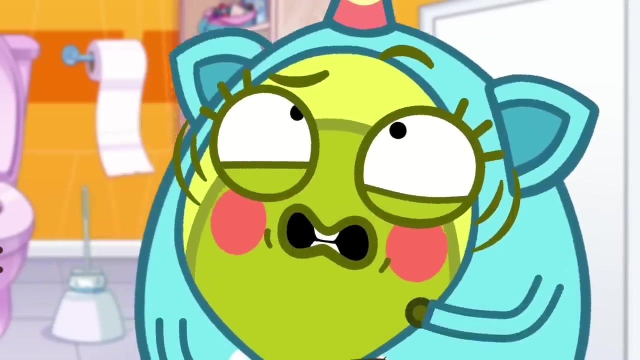 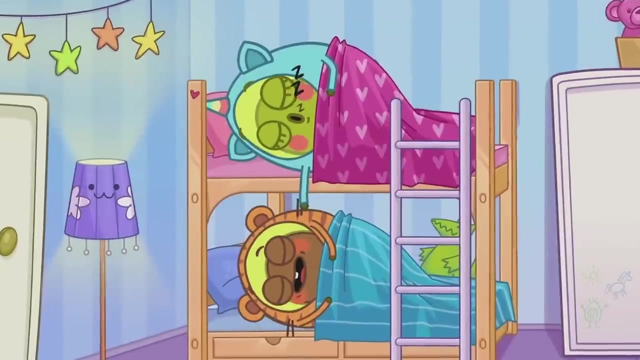 Tata, Tata, Huh, Hmm, Hmm, Hmm, Hm, Oh, Hmm, Toot, Toot-toot. No, no, Oh, toot-toot-toot, Toot-toot-toot, Toot-toot-toot. 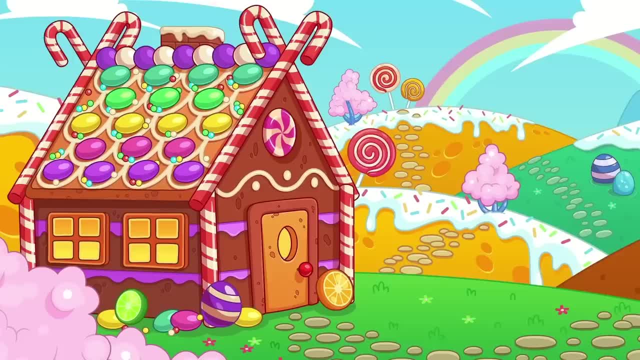 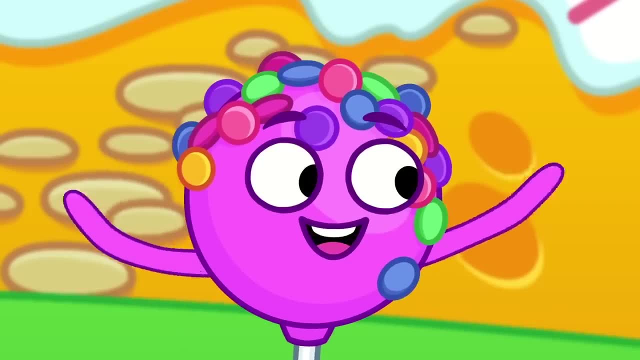 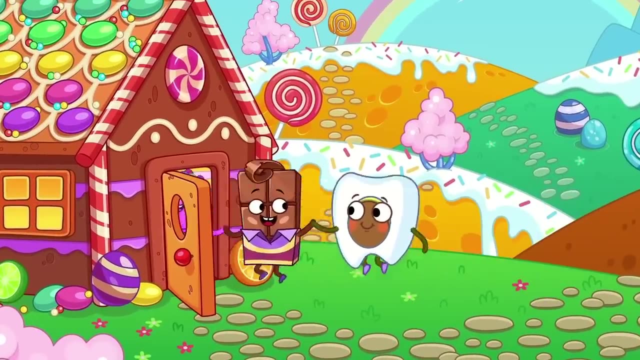 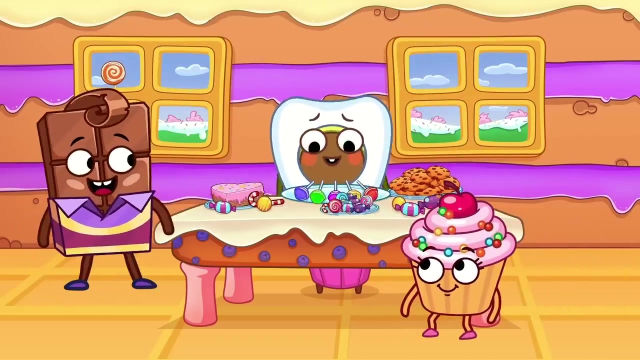 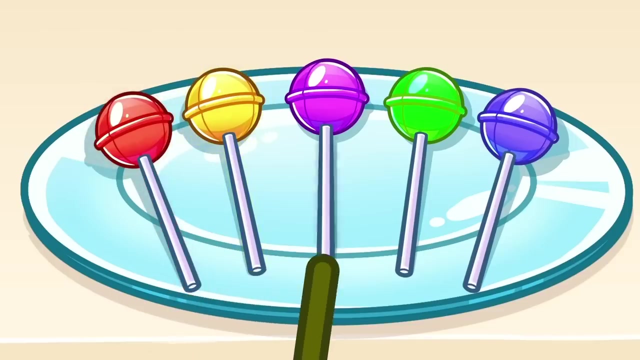 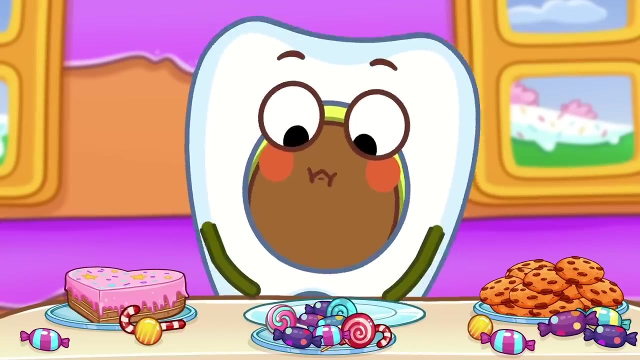 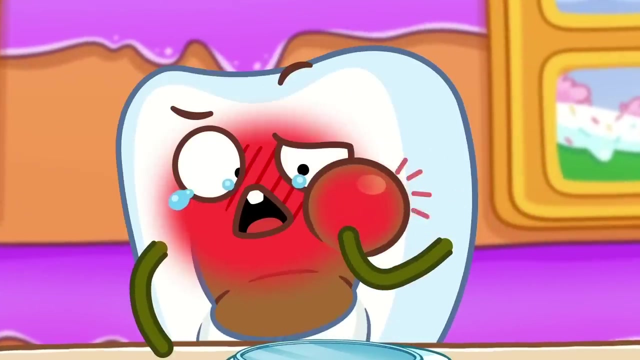 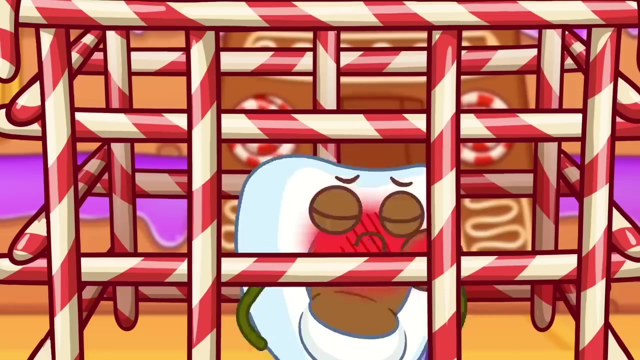 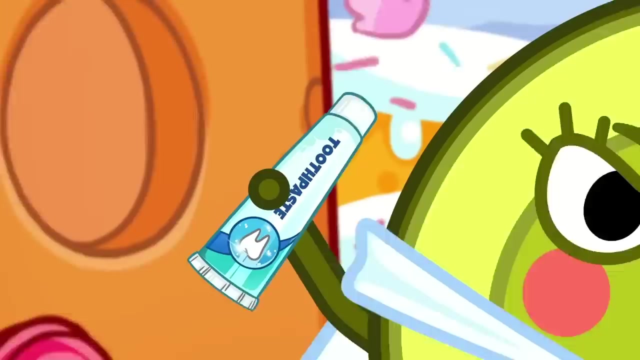 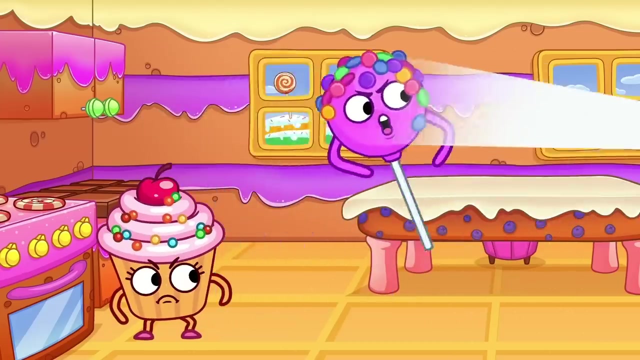 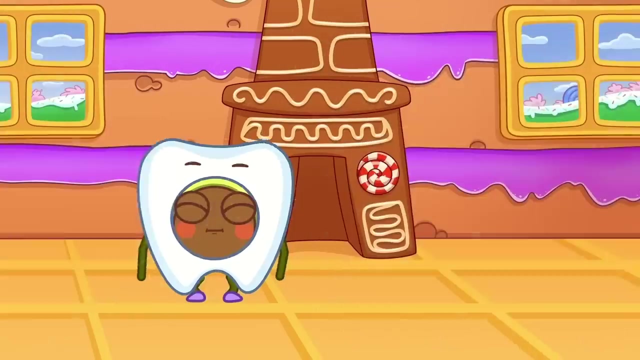 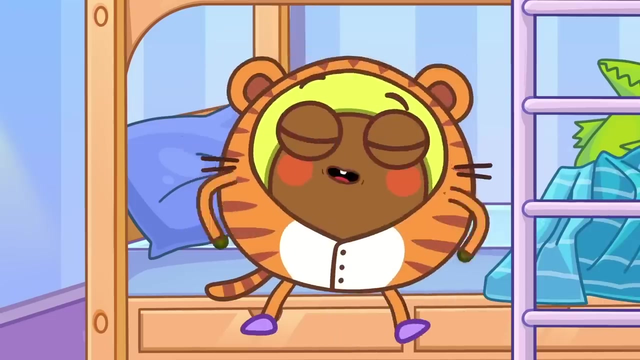 Hi, Toot-toot-toot, Toot-toot-toot. Red, Yellow, Pink, Green, Purple Pink. Popcorn. Red Purple Pink, Yellow Pink, Purple Pink, Purple Pink, Huh. 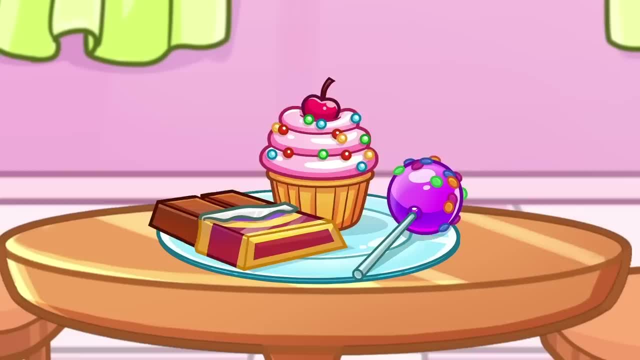